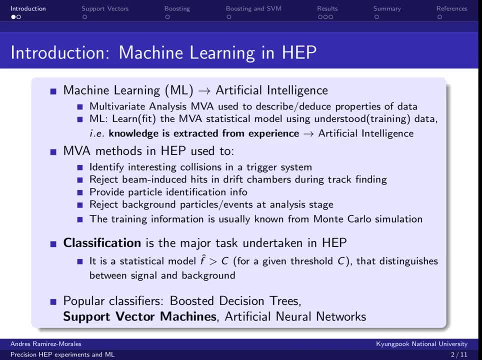 techniques have become very popular in many fields of science, but specifically in high energy physics. I list here the most important application of machine learning. For us, the most important one is the rejection of background against signal events when we want to do a measurement or analysis or physics. 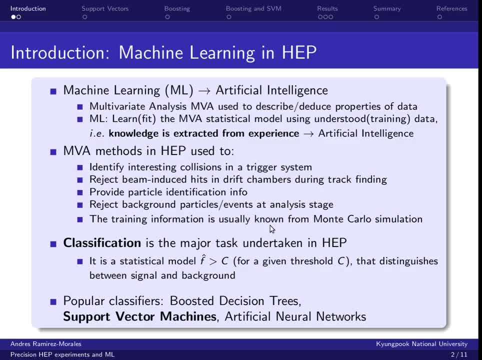 analysis and luckily we have that the training data usually can be known by Monte Carlo simulation. So the classification is building a statistical model that is capable of distinguish between signal and background, given a threshold, and the most popular classifiers that the people have been using recently are: 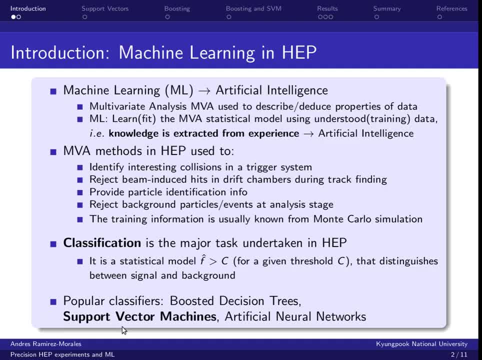 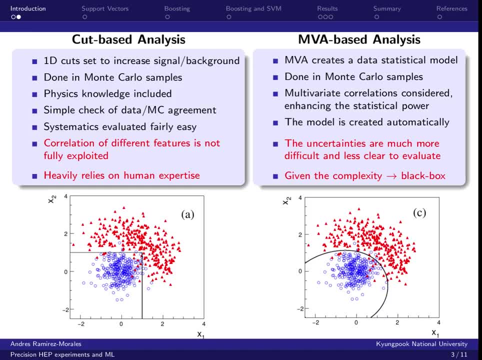 the boosted decision trees, artificial networks, and for this work we are going to treat the support vector machines To give a more clear idea of why the people are using more and more the MBA analysis. I make a comparison here between the more traditional cut base analysis and the MBA analysis. So basically in this: 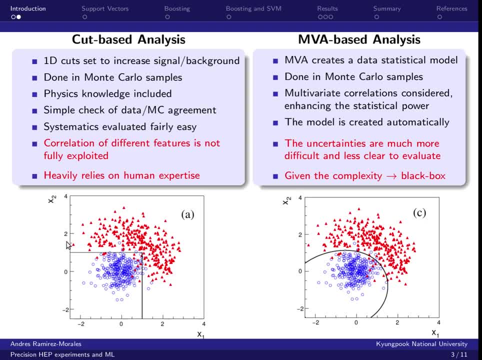 plots we can see how both of them are done. so in the cut base analysis we do one-dimensional cuts. here one cut, one cut, and we we try to discriminate between the, the, the signal and background, and here the same. here we can see that the classification is better because the MBA method uses the correlation between the. 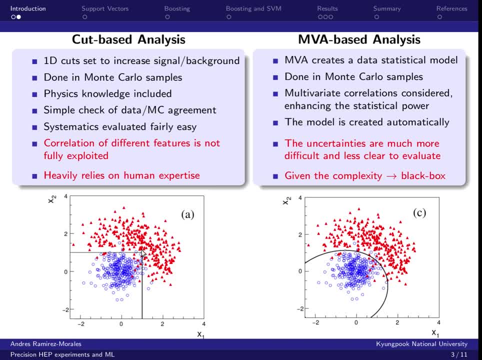 variables, while here only is one-dimensional. cuts that rely very heavily on human expertise are done. so the main advantage of using cut bases that the systematics are very easily evaluated, whilst in the MBA method are more difficult to evaluate. but at the end the people are preferring these methods because the statistical power is much. 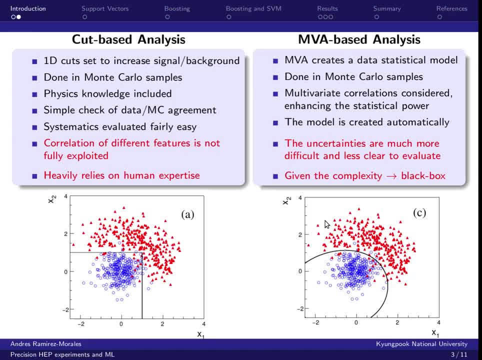 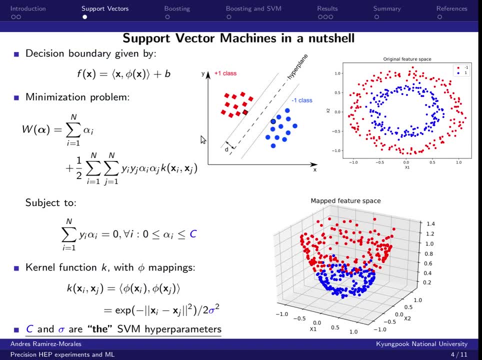 better using the MBA. so this is very helpful when there is a search of a very small signal in a detector. Okay, so we pick a definite support vector machine algorithm because it gives us a lot of nice properties. so at the end we want to do the same task, which is: 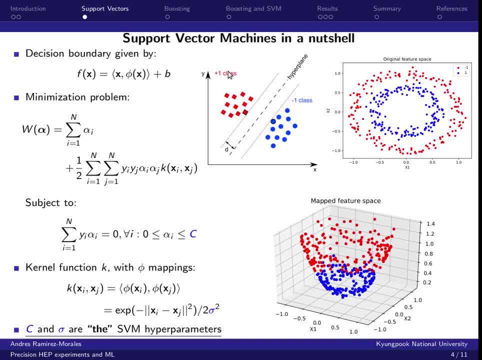 classifying between two different classes here- plus plus one and minus one- and the idea is to build a boundary. here is just a line, because we are dealing with linearly separable data. that follows the optimization problem to maximize this distance and this is done by building this equation subject to: 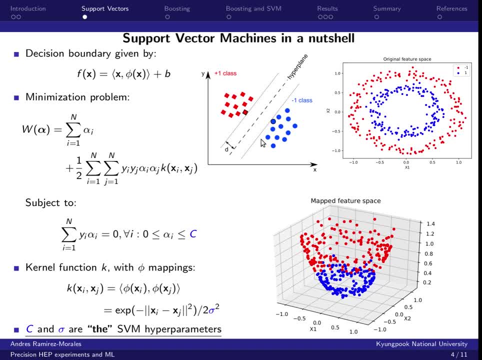 these conditions right, but in real life we don't have this kind of problems. we have something which is not linearly separable. so to solve that problem- but support vector machine does- is to do a mapping between the original feature space, which corresponds in this case to x 1 and x 2. 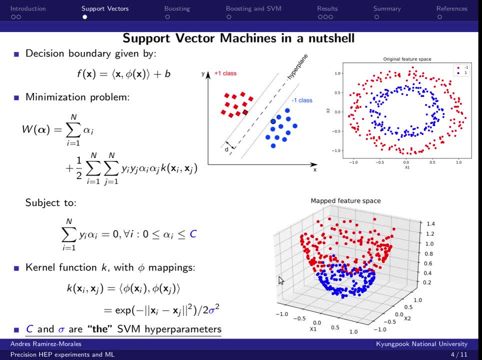 to a mapped feature space where the data can be separated with, with a plane. you can imagine here the plane that separates very well the data. this is done again. you see now a mapping and you see something which is called a assurance vector change, the kernel trick which enters here, and the most popular kernel that is been using it is the one. 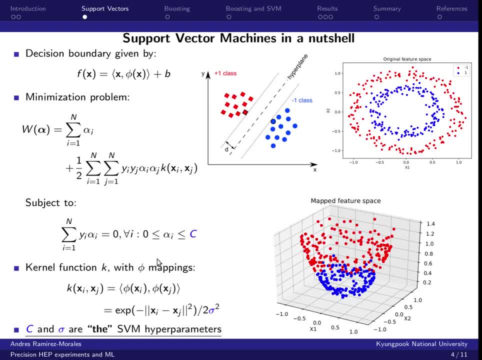 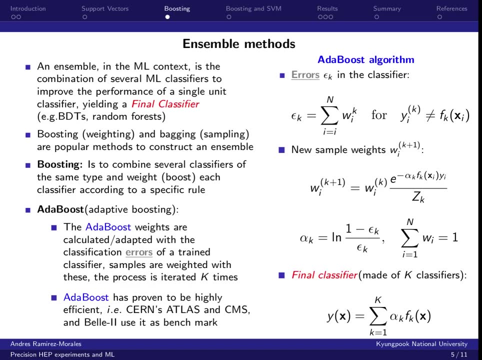 that we show in this presentation is the gaussian tree, the gaussian kernel and the parameters of this kernel and the support vector, machine, rc and sigma. now that we have defined which as which machine learning algorithm we're gonna use, we wanted to improve its performance, so the way 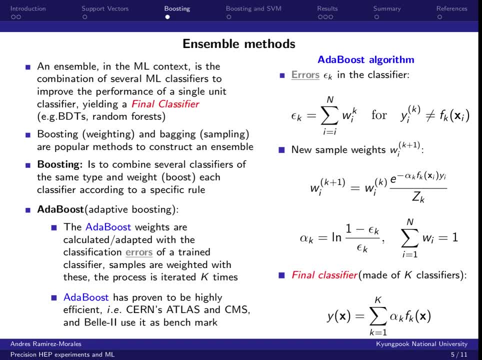 to improve it is is using ensembles method. so, basically, an ensemble method is a combination of many classifiers to yield a classifier which is stronger. and the way to construct this, uh, these ensembles is using boosting and bagging. here we focus on boosting, which is combining a classifier using weights, or boosting according to a specific rule. here we focus. 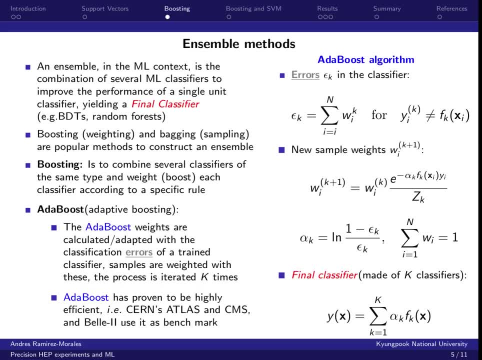 to using the other boost, because it's the one which is used by the high energy experiments and basically here, uh, the uh rule to do the boosting is based on how the errors of the training classifiers- these are the training classifiers- behave with respect to the known classifiers. 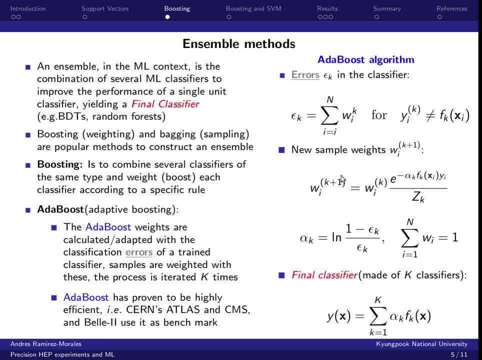 here we, we build the weights, uh, the errors. then we build the weights, and here we build a score. we repeat this procedure and at the end we get a final classifier, which is a linear combination, uh, which is weighted by these coefficients which depends on the errors. so here we're. 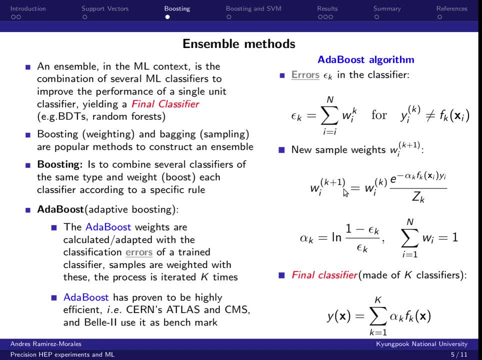 going to use the same method. we have a number of k classifiers. this final classifier, it's expected to be better because it is a voting procedure, so it takes uh, the different features in a different way. so so we have a stronger classifier now. why combine support vector machines and adaboost? 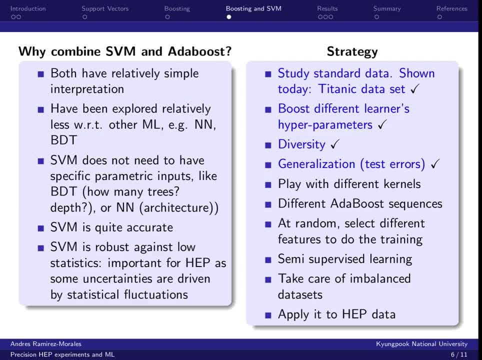 okay. the first reason is that both of them are simple uh to interpret, so this helps to follow systematic uncertainties also. both uh, especially support vector machines, have been been explored a lot with respect to other machine learning like bdts or neural networks, and probably the most important one is that support vector machine doesn't need a lot of expertise to have. 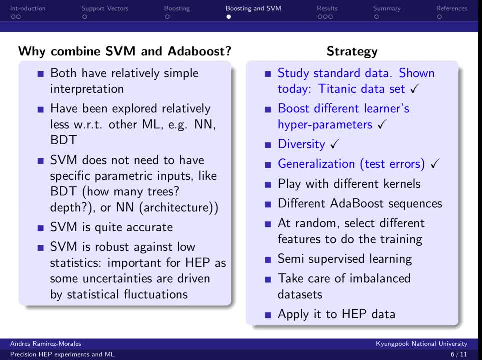 a nice classifier with, for example, if we compare with bdts or neural networks. you have to be very careful of how to build your classifier and also the support vector machine is quite accurate and finely calibrated so it can deliver a workload faster than other bdts or neural networks all. 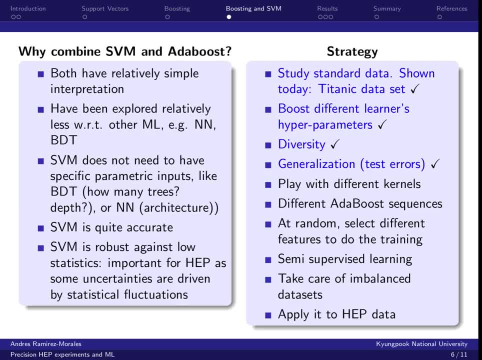 And finally, the support vector machine is robust. allow a statistic, and this is very important because in high energy physics some uncertainties are driven by statistical fluctuations and this basically tells the precision of our measurement Here. outline on the right the strategy of how to improve the support vector machine. 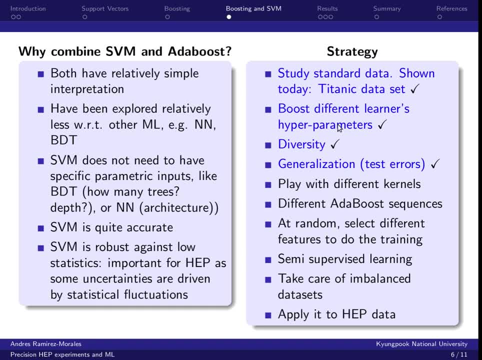 or how to do it Here. only four steps are presented today, and we study standard data that practitioners of machine learning use. Today I only show the Titanic data set. The second step is to boost a different hyperparameters, in this case the C and the Sigma, that we show. 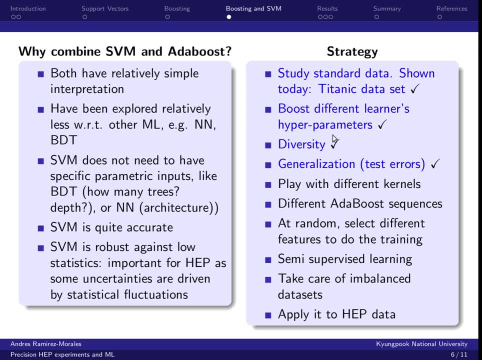 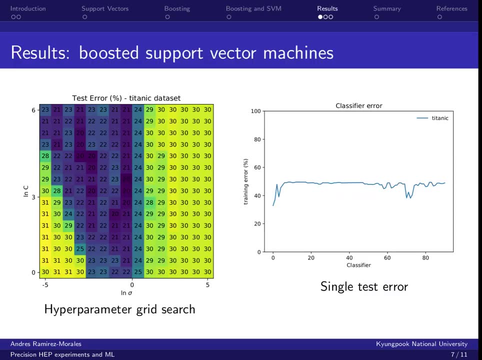 in the previous slides. We also take care about the diversity, to check how different each classifier is with respect to the others, and we get the test errors when we apply the training, the trained classifier, to test samples. Okay, let's jump to our results. So here in this plot, I show what I 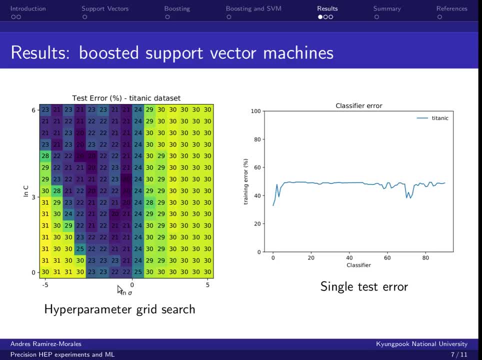 called the hyperparameter grid search. so basically, this is telling us how the support vector machine behaves with respect of the different Sigma and C hyperparameters. So this actually is a very nice to see, because we were expecting that the most important parameter is the Sigma, and this is exactly what we are seeing. so, for example, here you 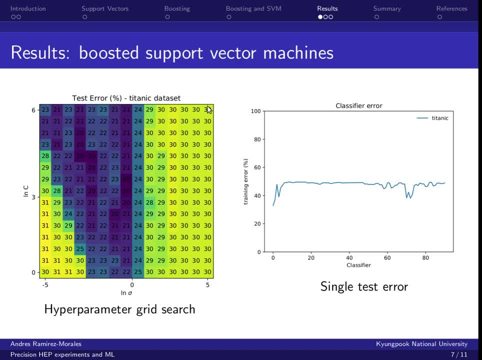 can see that if we keep one Sigma constant we have the same test error, but if we vary the Sigma We have some, some, some changes. this line, this part, actually correspond to some overtraining, which is when we over, when the model fits very well to this statistical fluctuation.